When we were to look at a catchment for a hydrological year, then the storage at the beginning of the hydrological year, meaning that the same amount of water is stored in the catchment. When we were to look at a catchment for a hydrological year, then the storage at the beginning of the hydrological year, meaning that the same amount of water is stored in the catchment. 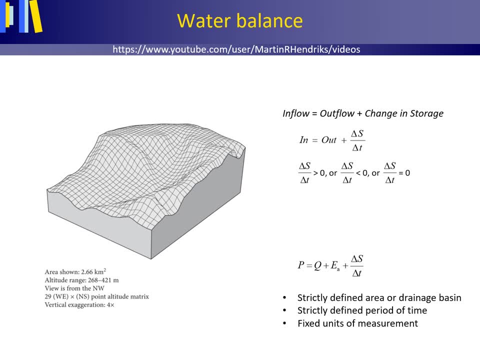 Now let's look more specifically at the Kriebsbach catchment. We assume that there is no leakage. The incoming term inflow is the precipitation P and the outgoing terms are the discharge Q at the outlet point and evaporation Ea from the catchment. 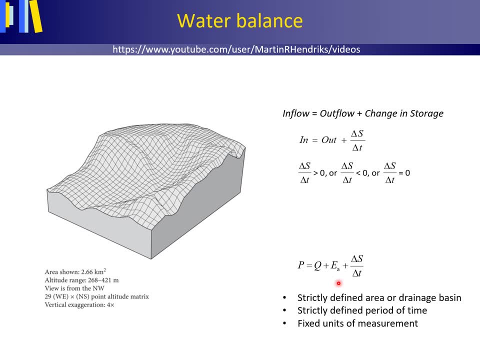 Inflow equals outflow plus change in storage: Delta S over that period of time: Delta T. There are some rules that you should always abide with. Always use a strictly defined area for the water balance, which, in this example, is the drainage basin or catchment. 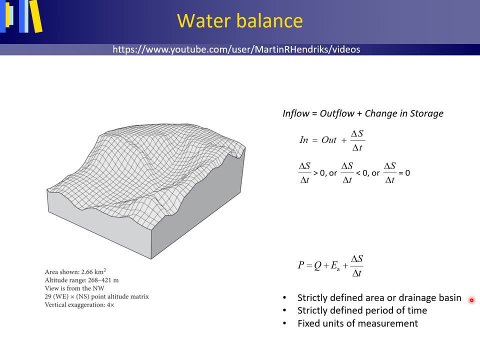 For instance, you cannot determine the amount of rainfall for a certain portion of the catchment and then determine the discharge rate. Always use a strictly defined period of time. If you have established the amount of rainfall for a certain day, you must use the discharge. 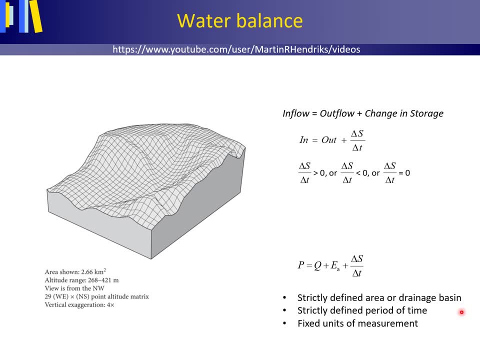 and also the evaporation and also the change in storage over that same day. In essence, you always have to use volumes of water for the same strictly defined period of time. Thirdly, always use fixed units of measurement. For instance, you cannot insert precipitation in mm per day and discharge in m3 per day. 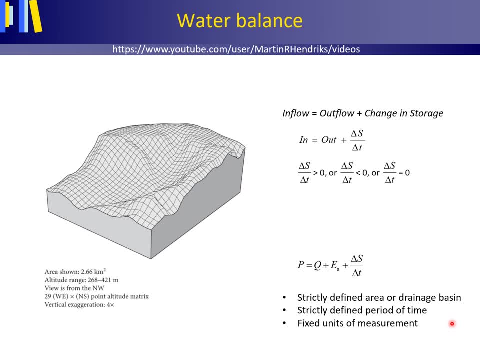 So you must either rework rainfall from mm per day to m3 per day, or you must transform the discharge from m3 per day to mm per day. What links these values? Let's take a look. First of all, we need to know the flow rate. 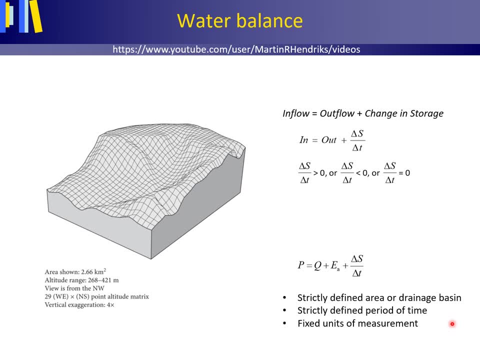 We need to know the values of mm per day and m3 per day, the catchment area in m3.. If you want to go from m per day to m3 per day for the precipitation, multiply by the catchment area in m3..